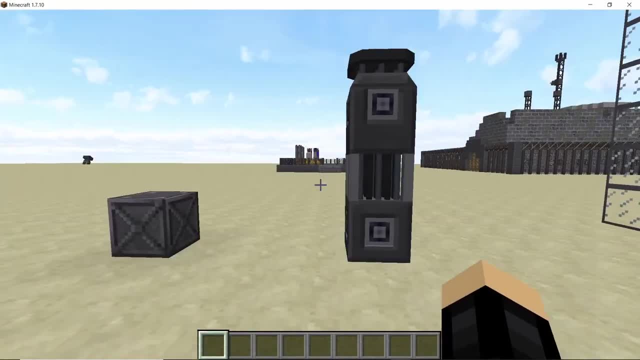 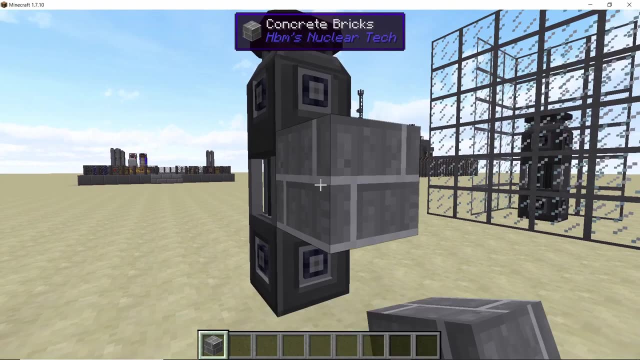 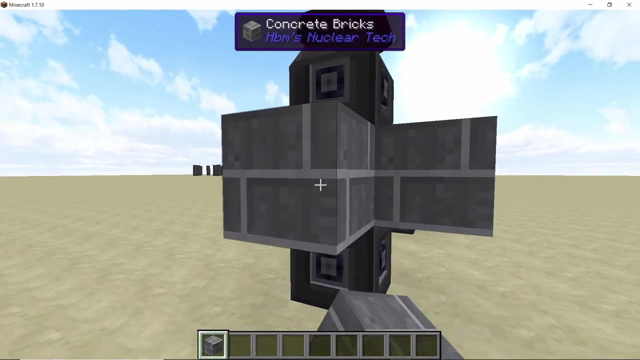 into this reactor. But wait, there is more. Now, when you start the reaction, it is going to give off the atmosphere. So in order to protect this, you need to cover the open sides of the nuclear reactor with concrete bricks, and if you do that, the radiation will be contained. But this has some 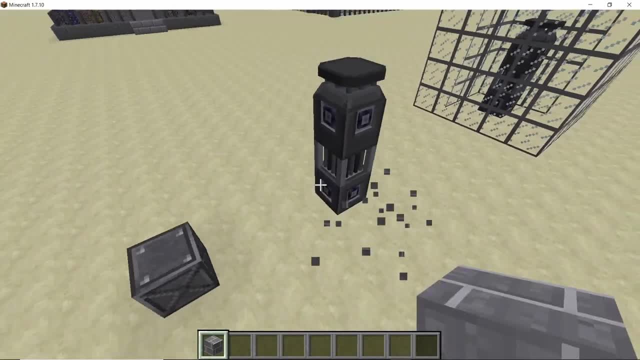 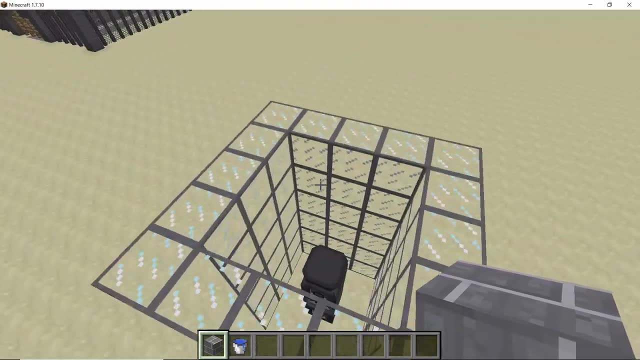 disadvantages, and I'll tell you why in just a minute. So, before that, let's take a look at another thing that you can do in order to control the radiation, which is also used in real life, by the way- You can build the entire nuclear reactor underwater. So, as you can see, here I have placed 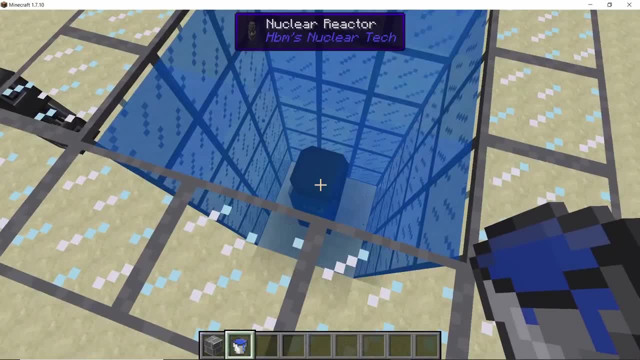 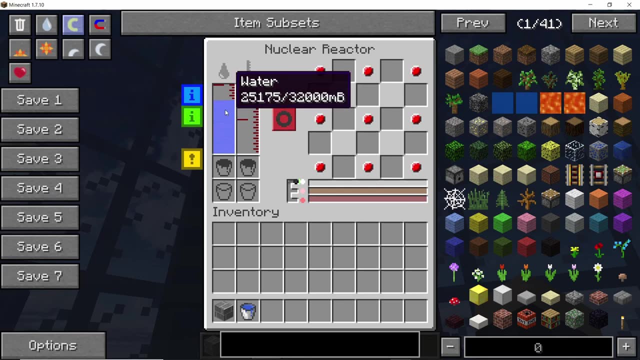 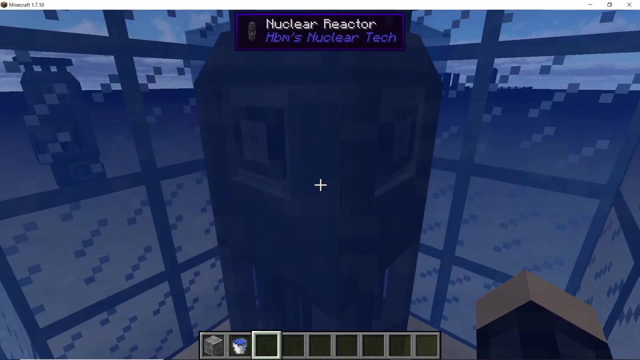 the nuclear reactor And I covered the entire periphery of it with water. And now, if I go down and click on the nuclear reactor, you will see that water will start filling up and this water is never going to go up. So, by the way, you need not supply any water to this nuclear reactor And also this water will not let. 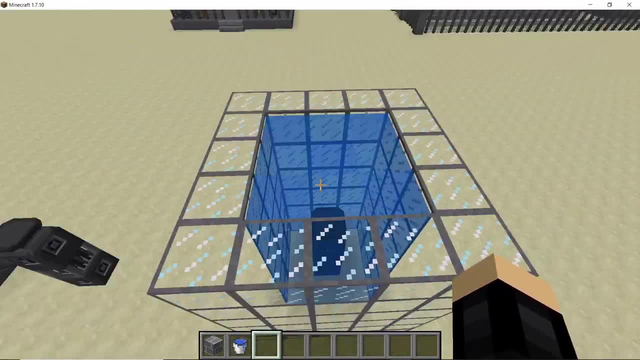 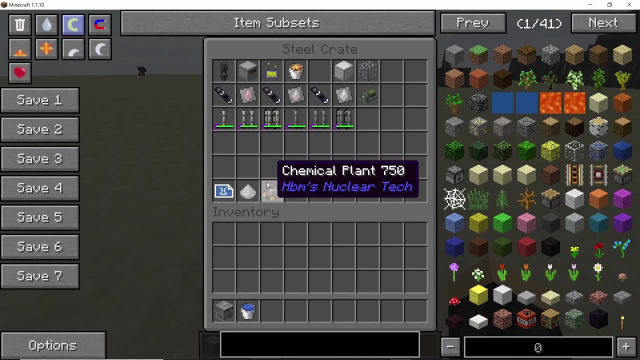 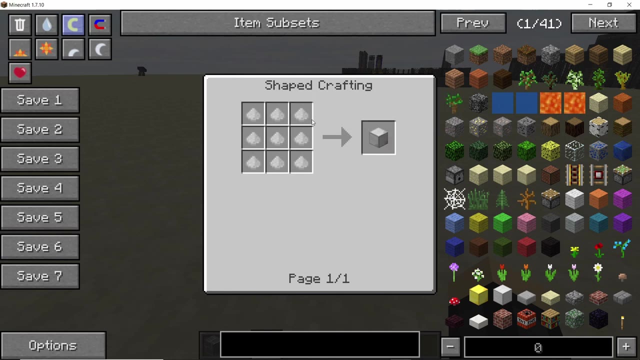 any radiation out into the atmosphere. So yeah, two for one. Now also, this nuclear reactor can produce infinite amount of coolant. You heard that right. This nuclear reactor can produce its own coolant, and that is something that is. only you need to this small nuclear reactor, And for that you need one single block of nitre. So when you take a block, 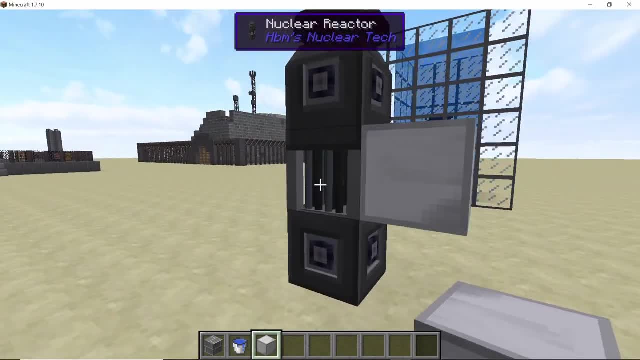 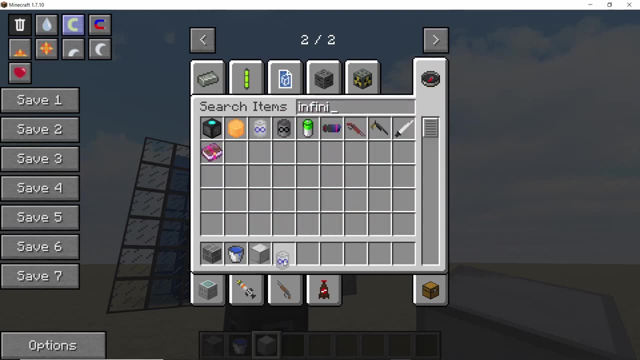 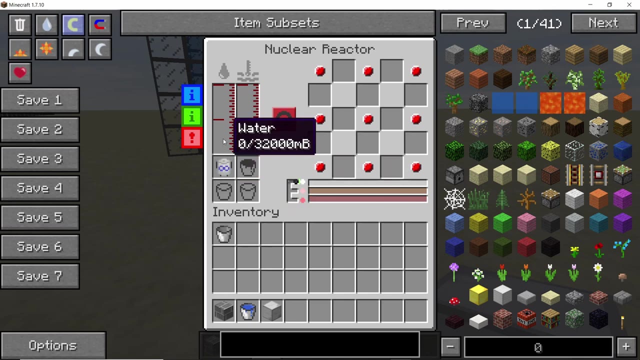 of nitre and you place that block on any of the open side of the small nuclear reactor. And now that if I start placing some water in this nuclear reactor, So let me demonstrate that with an infinite water tank And if I place this water here, you will see that this nuclear reactor will start. 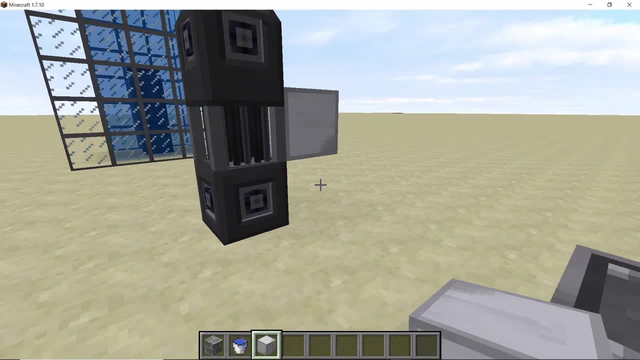 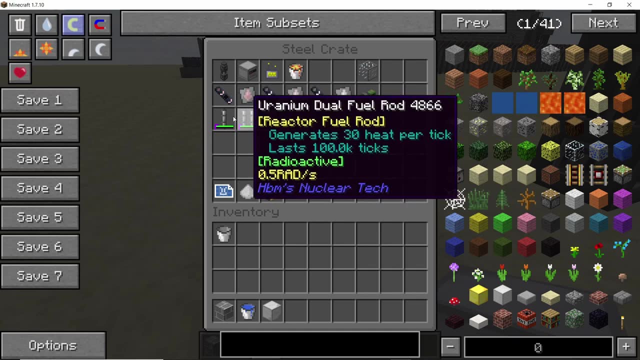 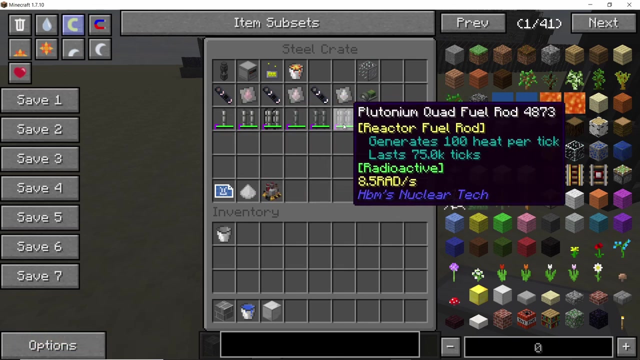 producing coolant. So yeah, infinite coolant Guys, no more need to produce any coolant or water. So now let's take a look at fuel, Uranium fuel rods and plutonium fuel rods. Now you can produce dual fuel rods or quad fuel rods. Both of them, or rather all three of them, will have different 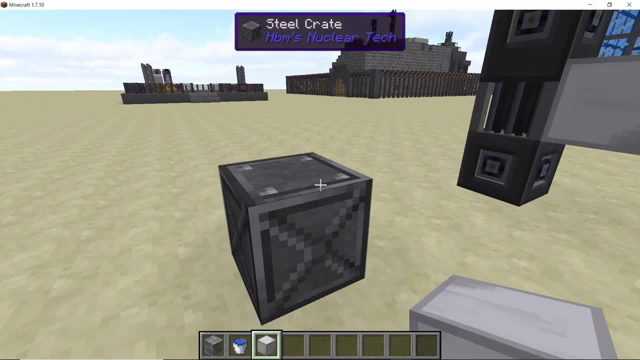 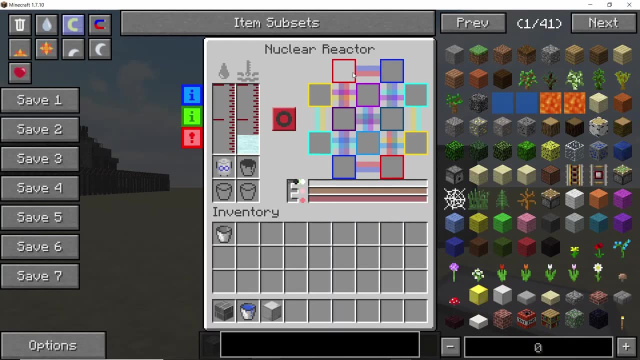 heat particles and they will last for nearly the same amount of time. But yeah, if you use the quad fuel rods, the better it is, And also, this is how you can place the fuel rods. by the way, The closer you place them, the more heat they are gonna produce, but the sooner they are gonna burn. 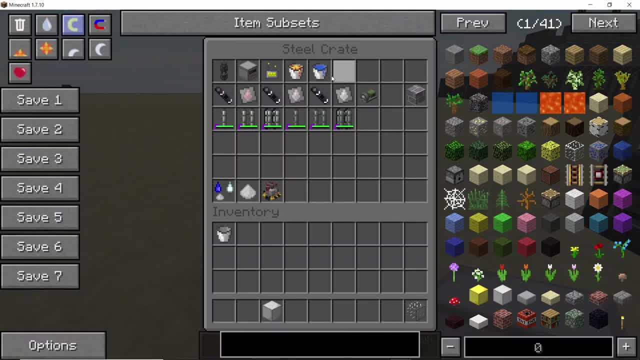 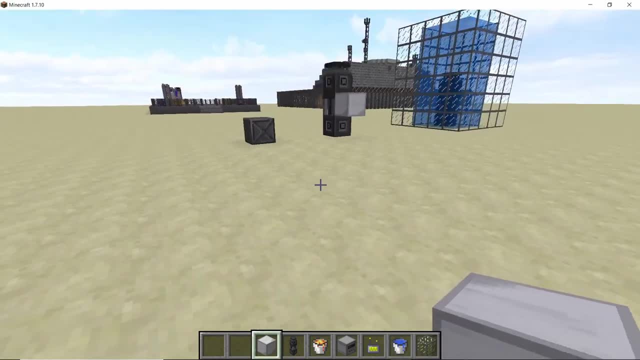 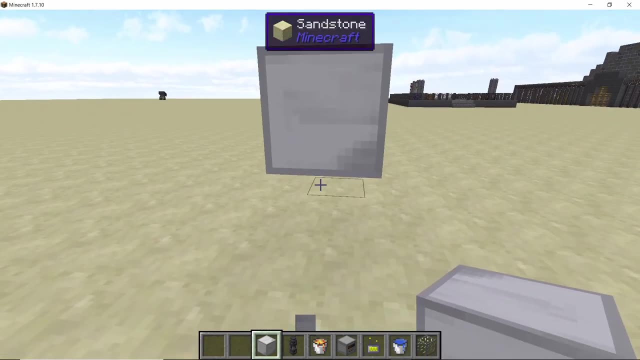 out. So make sure that you have that in mind. Now that we have covered all of this, let's quickly take a look at how to produce your very own nuclear power plant. So first of all, place down a block of nitre, one block away from the ground, and then, surrounding it, place down four nuclear reactors. 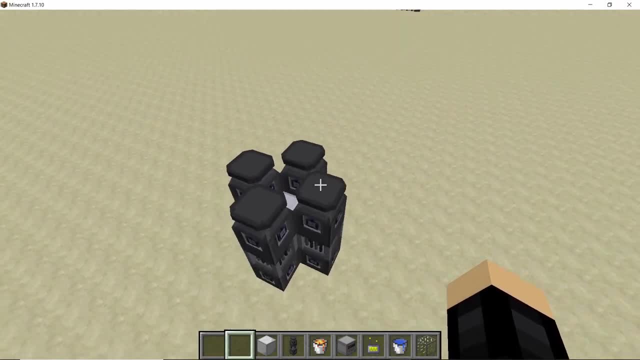 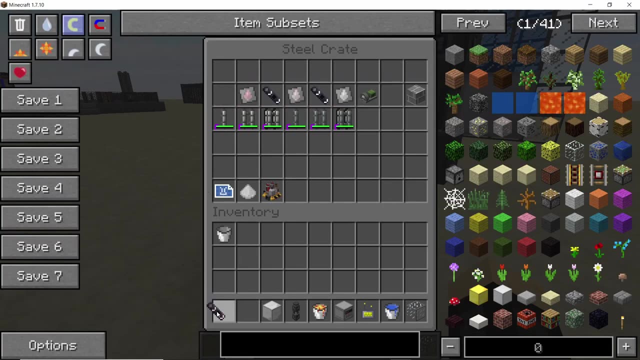 So that All four of the nuclear reactors will share this one block and they will produce coolant from it. This is the most efficient way that you can arrange the nuclear reactors. But if you don't have these many nuclear reactors, you can also put down one or two, whatever. 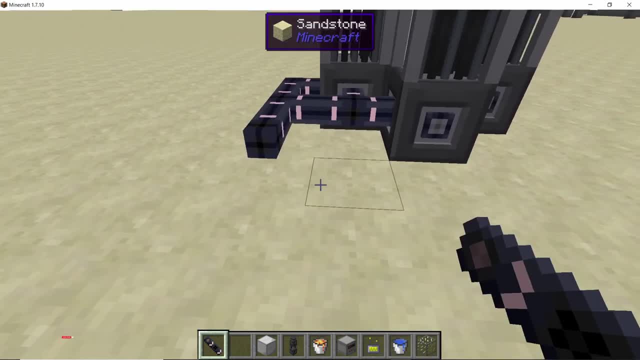 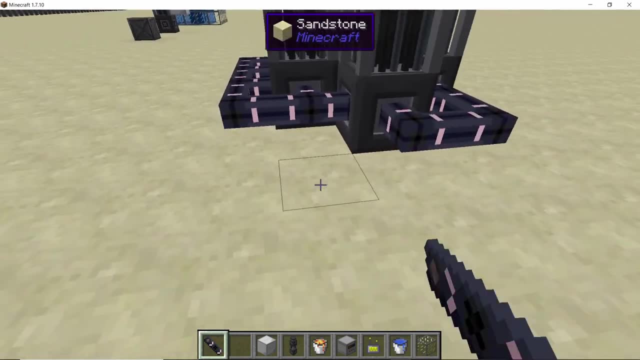 you would like Now, from each and every single one of these nuclear reactors, take out super dense steam pipes. and listen to this carefully: You need to take out the super dense steam pipes Now. it is up to you if you only want to produce dense steam or normal steam, but the reactor 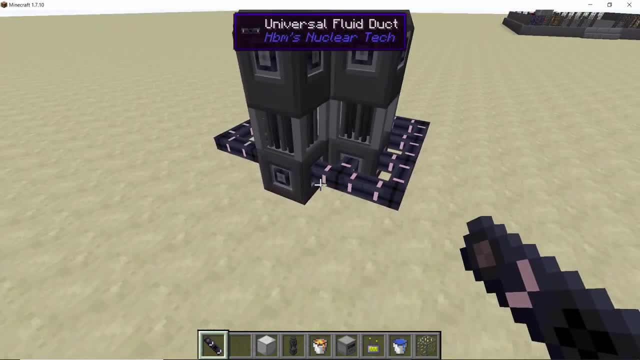 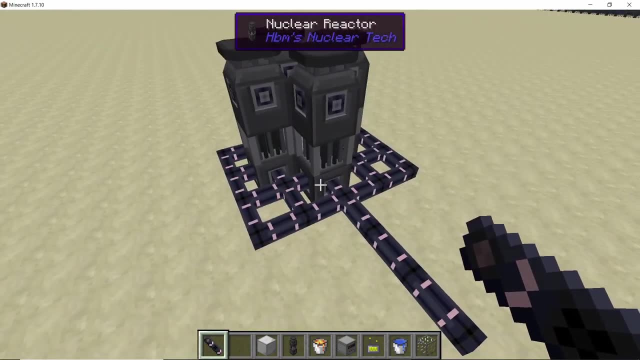 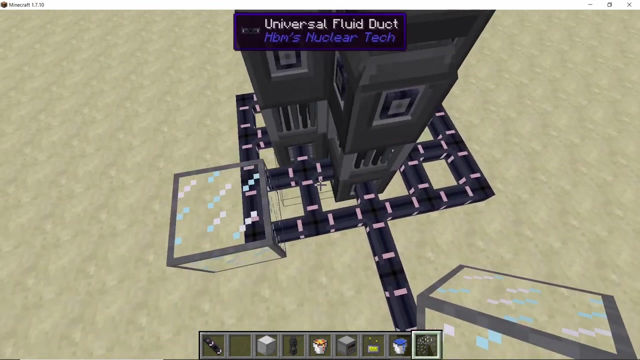 will work best when it is producing super density. So in this way, connect all the pipes on the bottom and take these pipes out, and we will connect industrial generators to it later. Now it's time to produce a section in which we are going to place water and also modifiers. 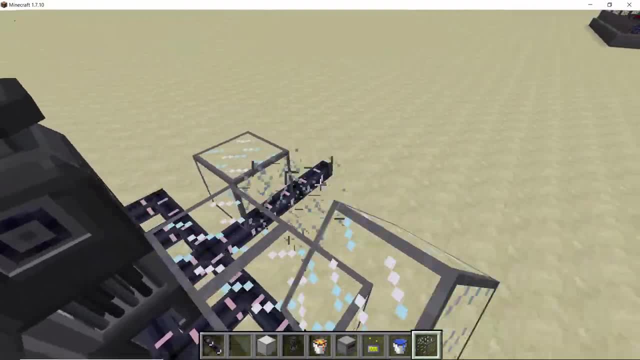 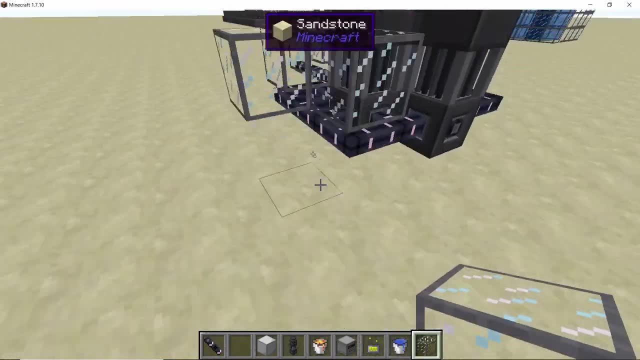 Now I will tell you what modifiers are in the later part of the video, but just make sure that there is a one block gap like this: There is a one block gap, There is a one block gap. There is a one block gap between the open end of the nuclear reactor and the place where 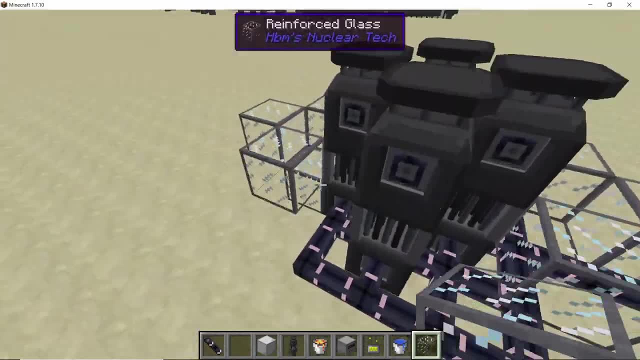 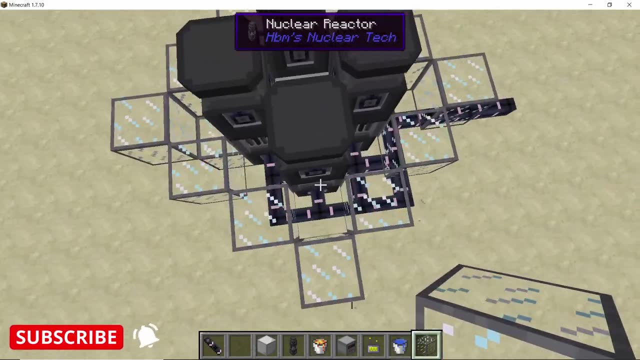 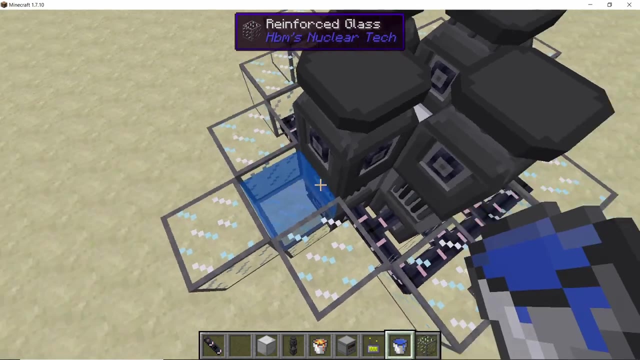 you are placing the glass, and wherever there is no ground place, some glass there. So now that I have covered the entire periphery of all the nuclear reactors with spaces like this and the pipes won't let any water out, start filling them up with water. 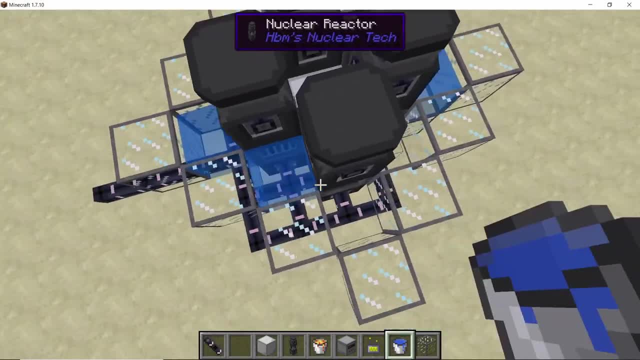 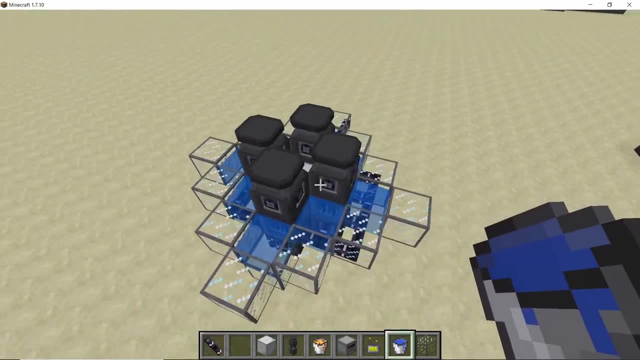 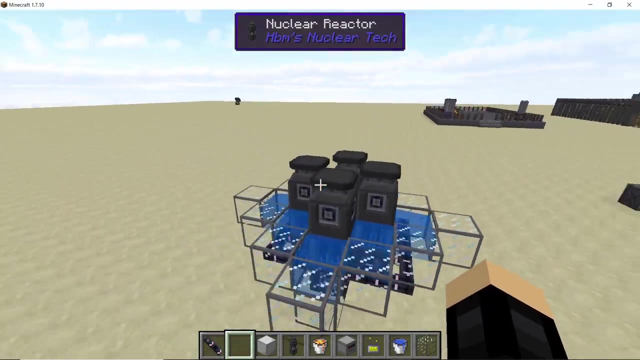 Now, when you do that, as you can observe, every single nuclear reactor has three phases exposed to water and one phase exposed to the niter block, So it can produce its own coolant and it has also infinite amount of water supply. So, as you can see, all the nuclear reactors are now producing water and coolant. 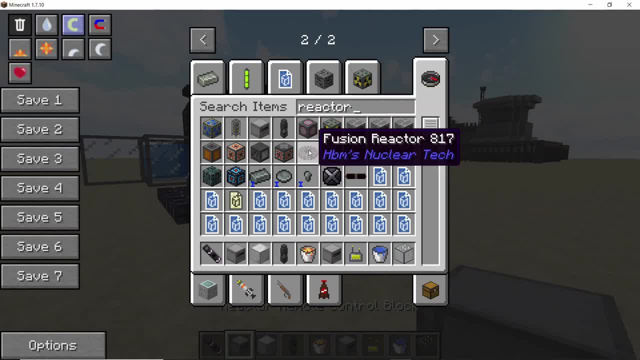 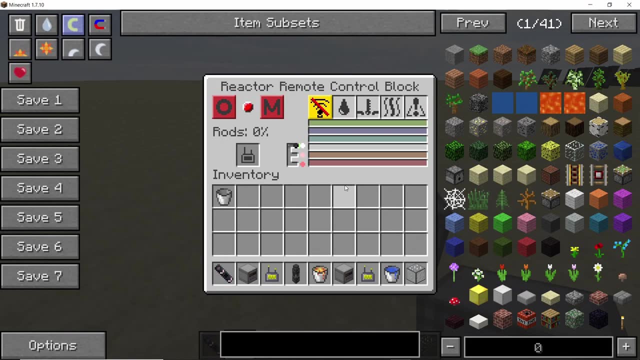 So, with that said, there is also one other thing that I want to show you guys, which is the reactor remote control block. Now, in order to make this work, you are going to need the remotes for this and the number of power plants, or basically the number of nuclear reactors you have. that is the amount. 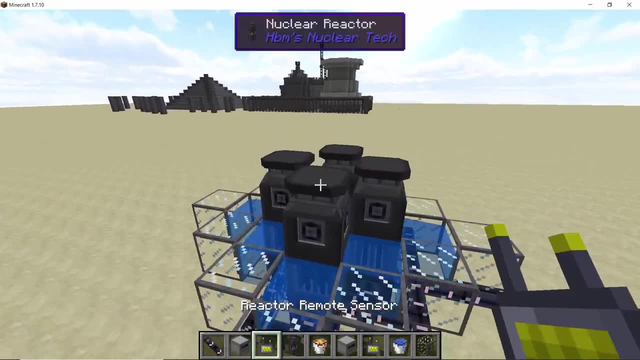 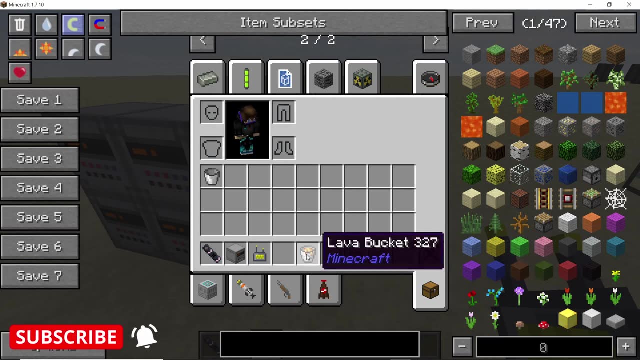 of reactor blocks and reactor remotes you are going to need. So here, as you can see, I am going to take four remotes because I have four nuclear reactors and I am going to assign each remote to a different power plant, oh sorry, different. 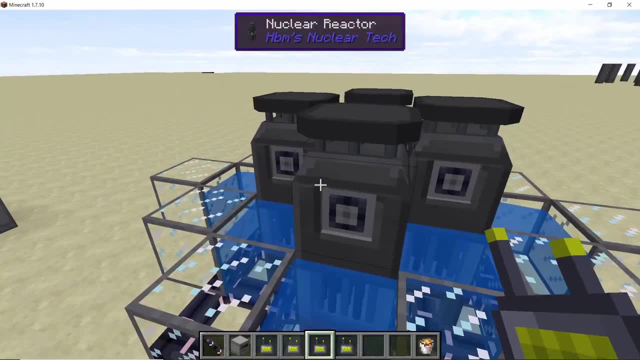 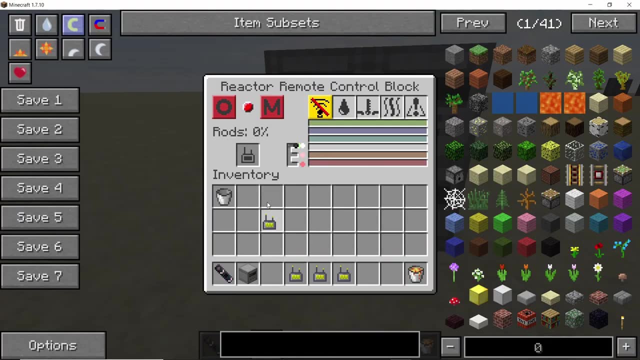 nuclear reactors one, two, three and four. You just have to right click on them, by the way, You just have to assign the position And now that when you will start placing them in the reactor remote control block, it will be assigned to that nuclear reactor. 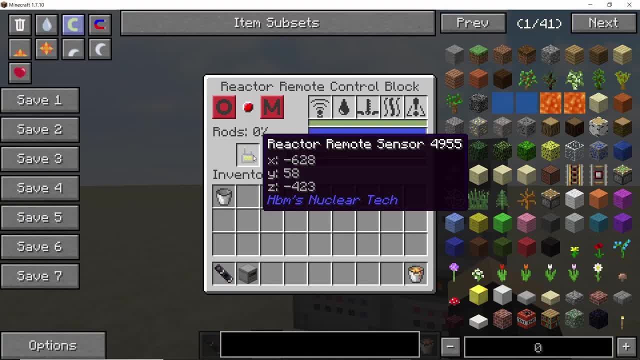 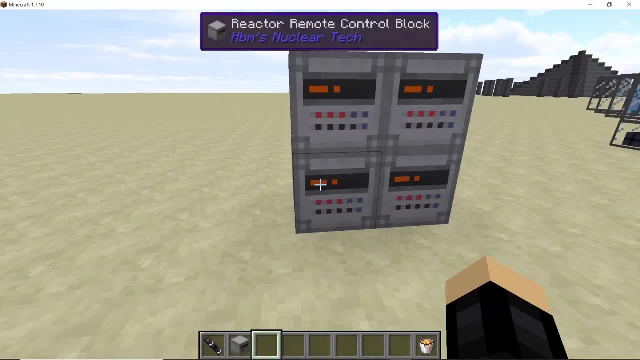 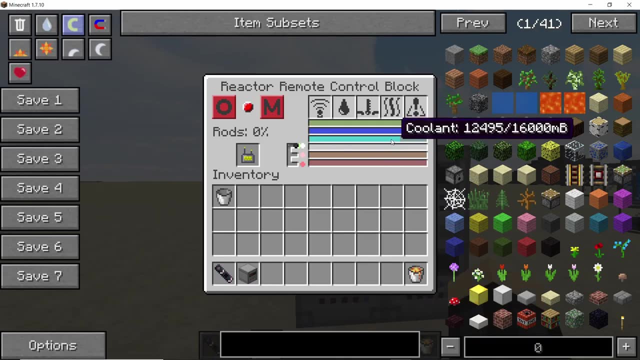 So, basically, you can control your reactors from far, far away. You don't need to be beside them in order to control them. And also, very one important feature about this reactor remote control block is going to be its automatic shutdown method. So, as you can see, now that the coolant is filling up, we are going to turn on the automatic. 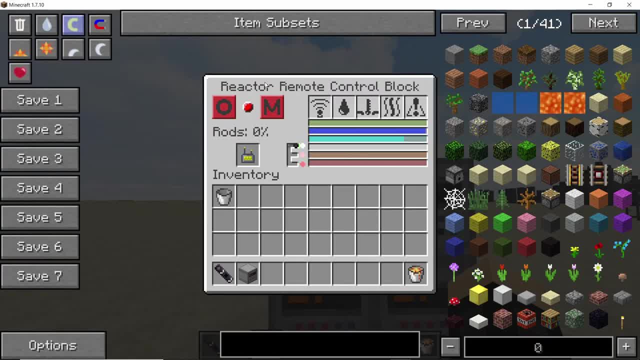 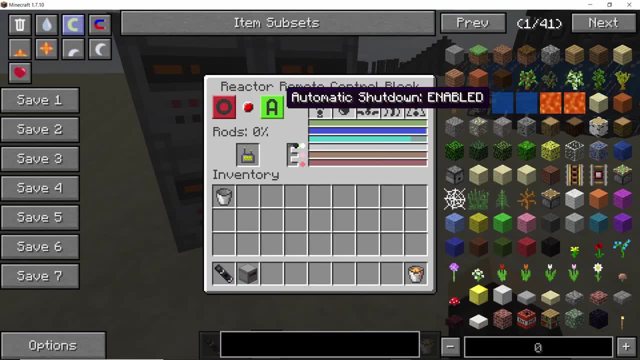 shutdown method. So this is the automatic shutdown for all the reactor remote control blocks. Now what the automatic shutdown will do is when it will detect that there is no coolant available anymore, it will automatically shut down the reaction so that your reactors won't melt down or they won't explode. 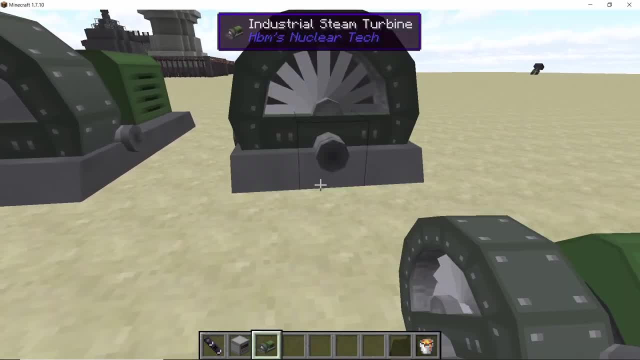 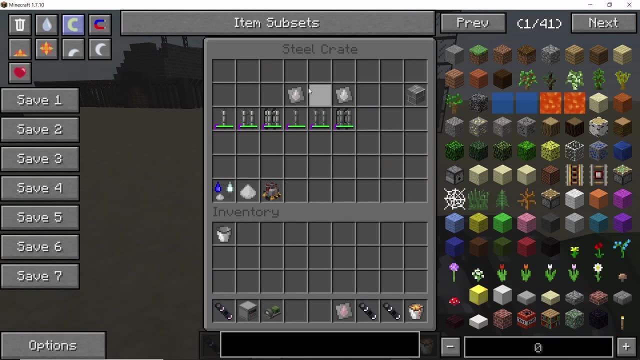 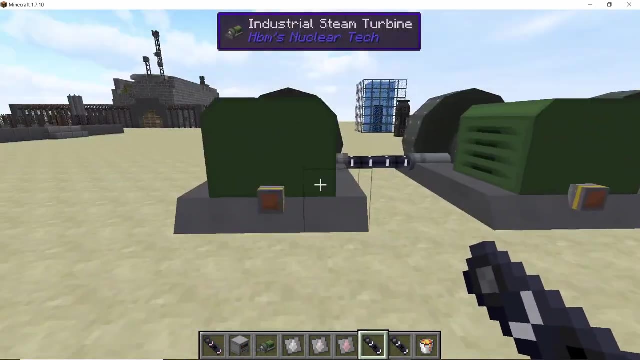 Yeah, that happens, So be careful while using that. Now that this is done, place down three industrial turbines and from the very first turbine it is going to take in the super density. Now We are going to get dense steam which goes into the second turbine. 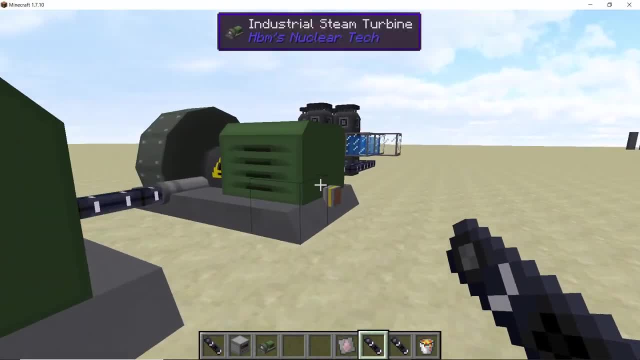 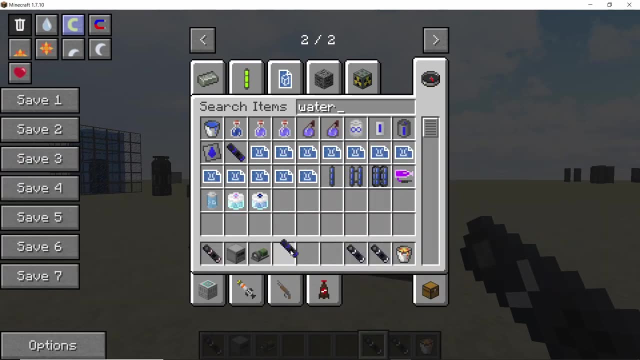 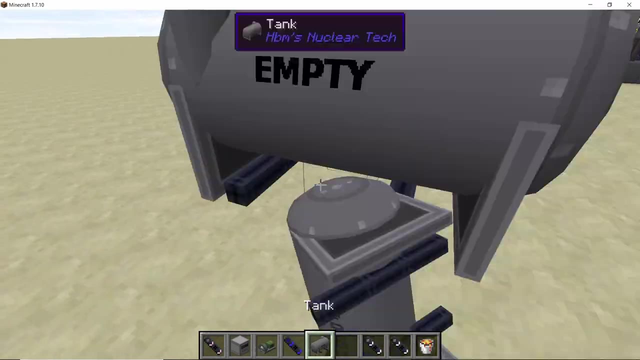 And finally, the third turbine will take the normal steam. So this is how it goes: super dense steam to dense steam and dense steam to normal steam, And that normal steam will then be converted into water, which then you can store in a tank, or even you can pump it up back into the nuclear reactors if you would like to. 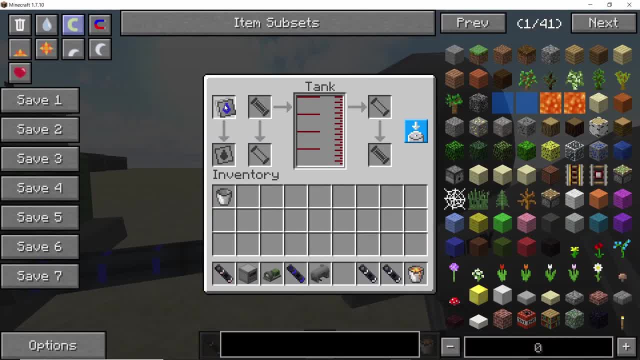 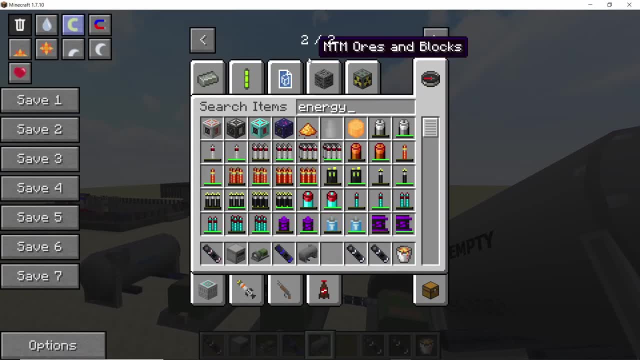 But I don't think that will be necessary, because by placing down three sources of water you already have more than enough water, And with that we are done, Thank you. So with this done, a nuclear reactor setup, or basically a power plant setup, is complete. 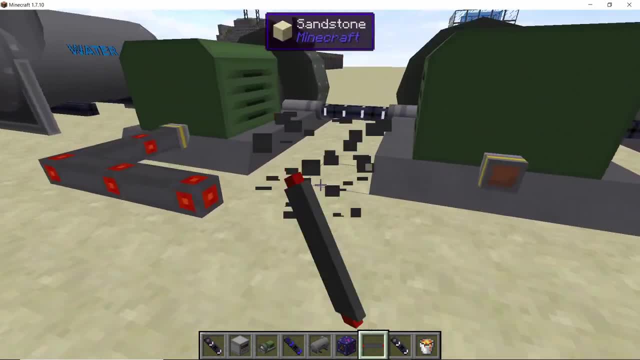 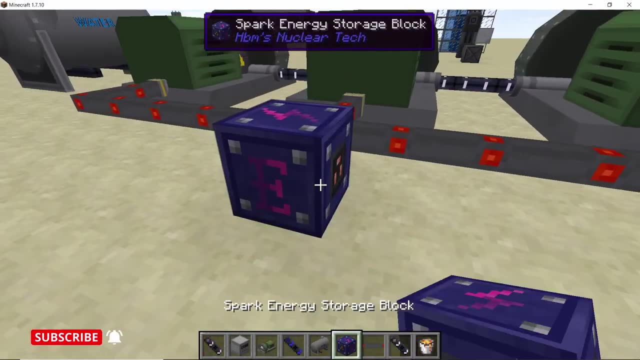 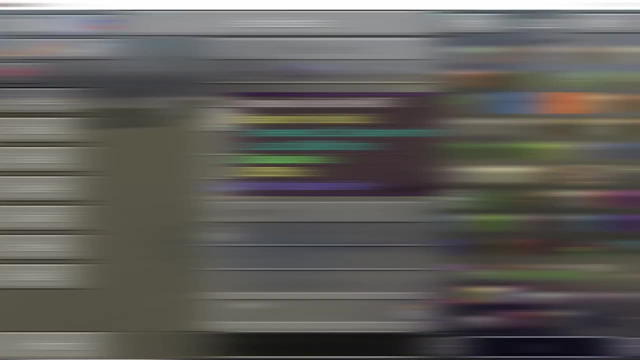 So the only thing remaining is to connect these industrial turbines via cable, And once you do that, yeah, the only thing remaining will be to place the nuclear rods and to start off the reaction. So we are going to start this thing with the most basic fuel rod. 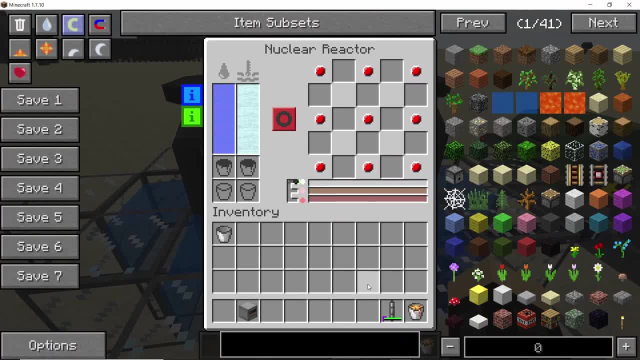 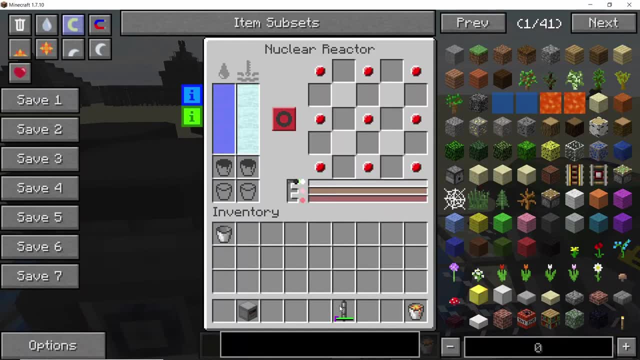 Which is a single uranium fuel rod, And we are going to see how much energy it gives us right. So, in order to start the reaction, you are going to need at least two fuel rods. You can have more, but you are going to need at least two to start the reaction. 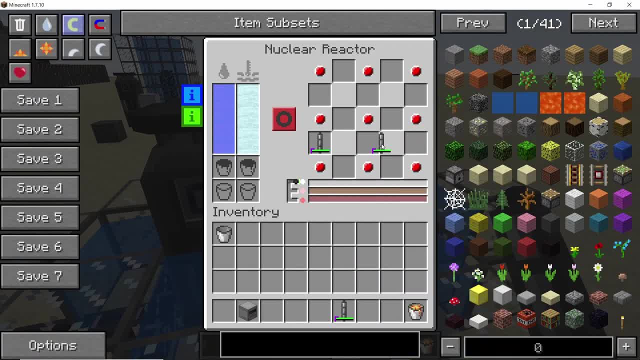 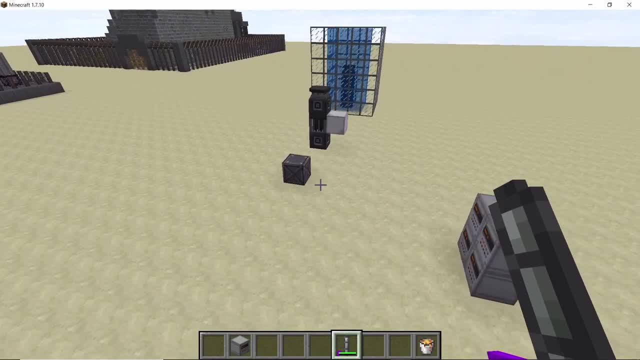 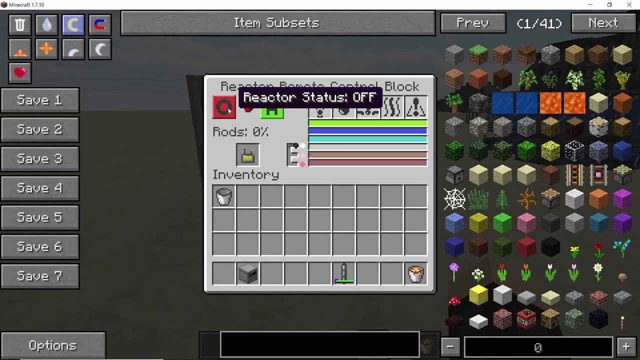 So place two nuclear fuel rods in each and every single nuclear reactor, The final one. And now, once that you have done that, it is time to raise the control rods and start the reaction off. So one, two, three, four, damn. 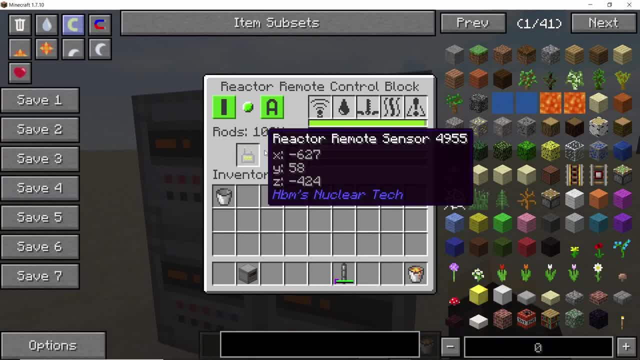 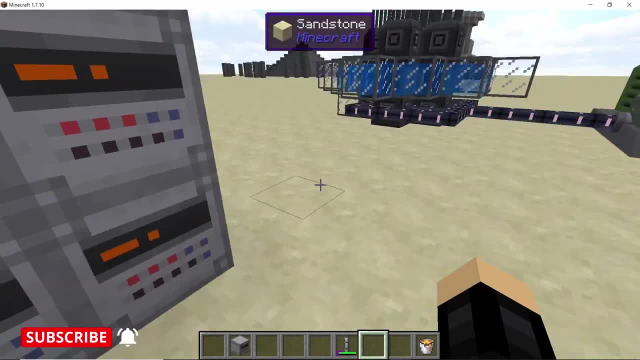 Look at how cool this looks. This is the best thing about these nuclear reactors: the control rods. And, by the way, don't forget to switch the compression to the third mode, which is the super dead steam, Otherwise your reactors will only produce normal steam and your this industrial generator. 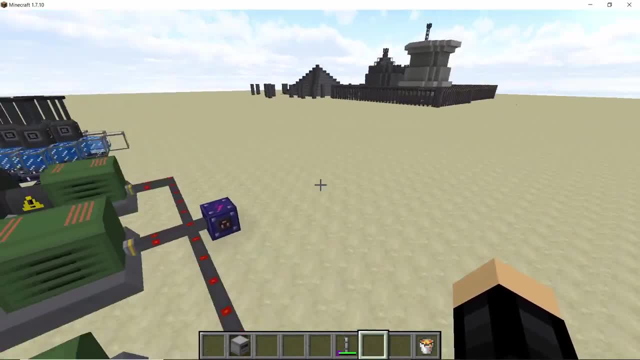 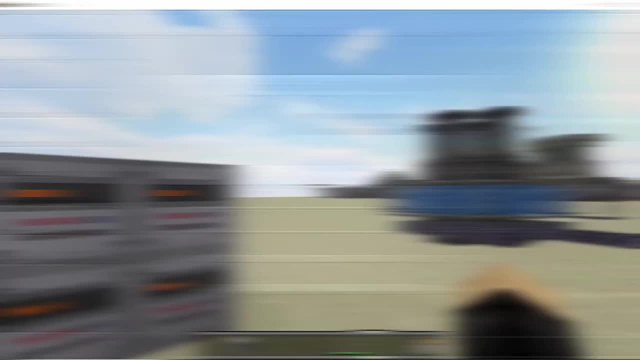 setup, it won't run. So, as you can see, we are getting energy And, yeah, look, we are already at 1 million Hg. Now there is another thing that I want to show you guys, which is the Geiger counter. 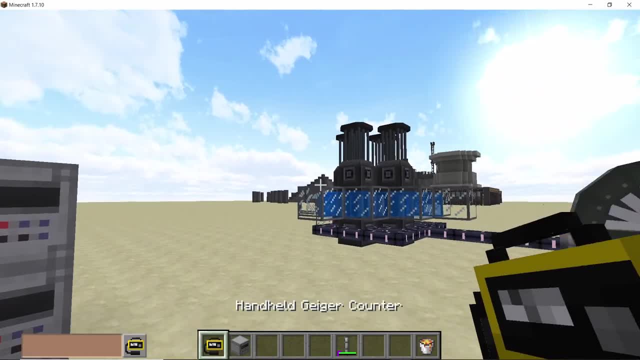 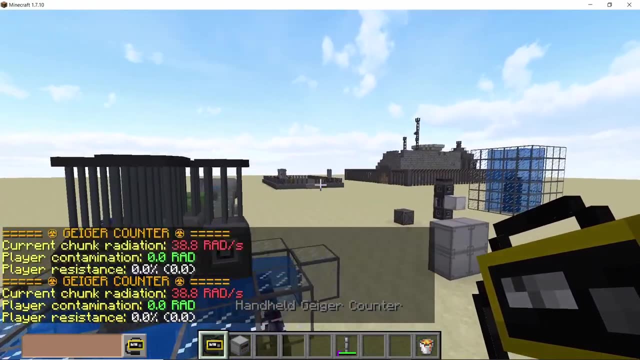 Now, if I quickly take the handheld Geiger counter and click at the radiation field, it is going to be, yeah, around 38 watts per second, And as you keep on going further and further, it's going to drop down to 35 or 32.. 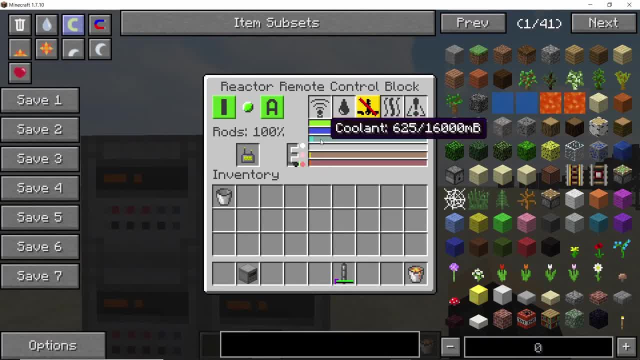 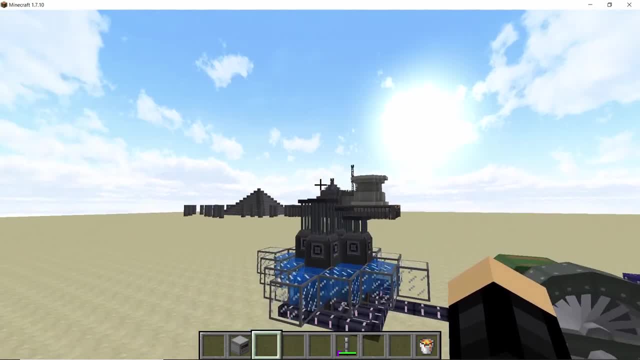 So, yeah, not very dangerous level of radiation, but still don't forget that. Okay, Okay, Don't forget to wear your hazmat suits Now, as the coolant runs up. as you can see, now the coolant has started running up. 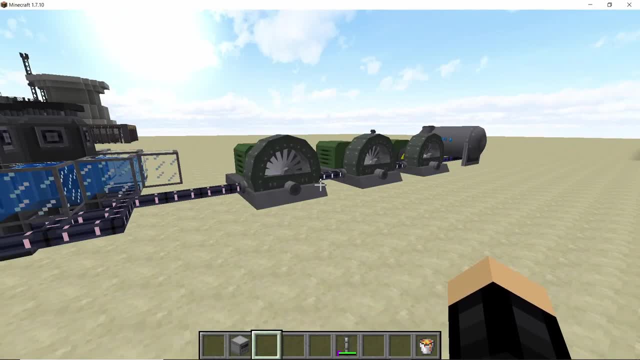 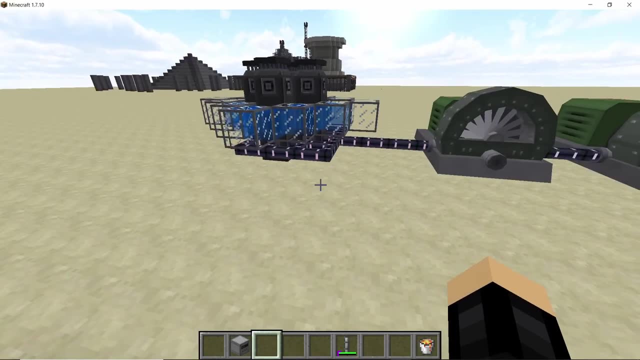 So our reactors have gone into automatic shutdown. Now the turbines have stopped rotating and the coolant has gone down, And as soon as the control blocks or control rods go down, the coolant will start filling up again. This is why the automatic shutdown was so important, guys. 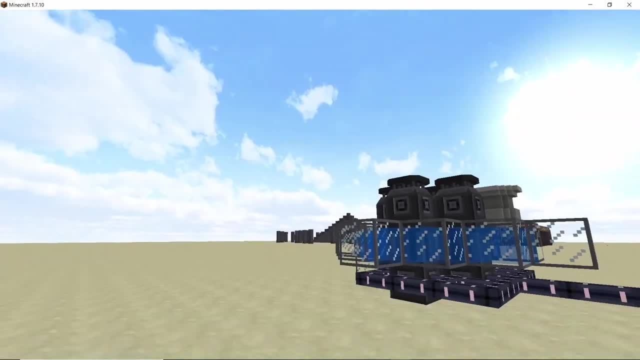 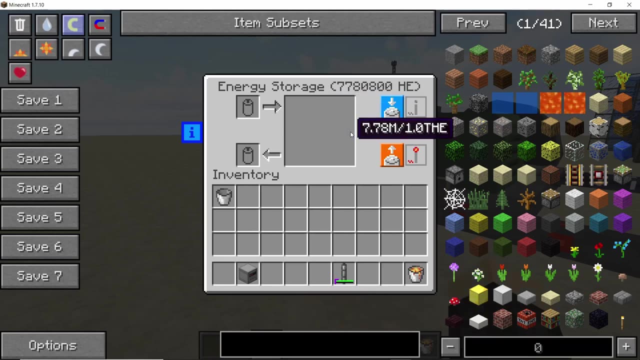 It will protect your nuclear reactor and your base. Now, finally, Let's take a look at how much energy we got from that operation: 7.78 million, So nearly 8 million Hg from one round of nuclear reactors running, and believe it, that is a. 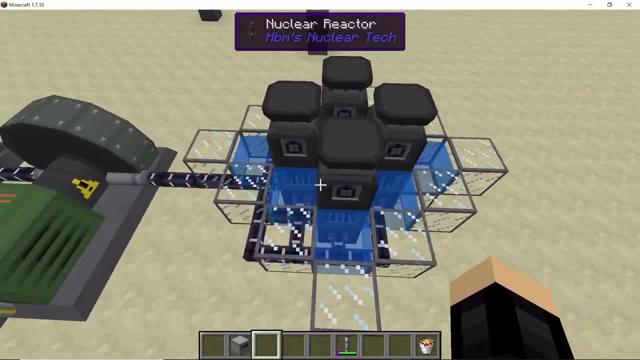 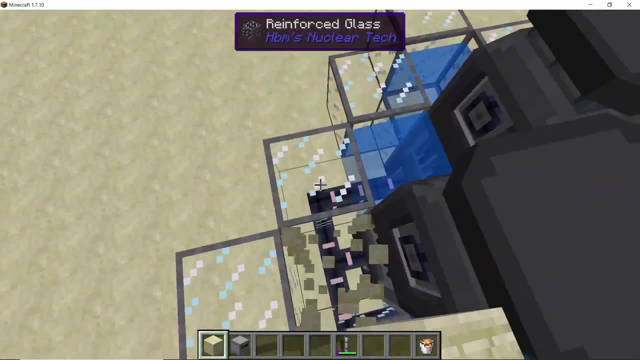 lot of errors, You still have a lot of efficiency left in those uranium fuel rods. So yeah, Now let's talk about some modifiers. Now, there are a lot of modifiers available and I am going to post a screenshot here which is available on the Wikipedia page. 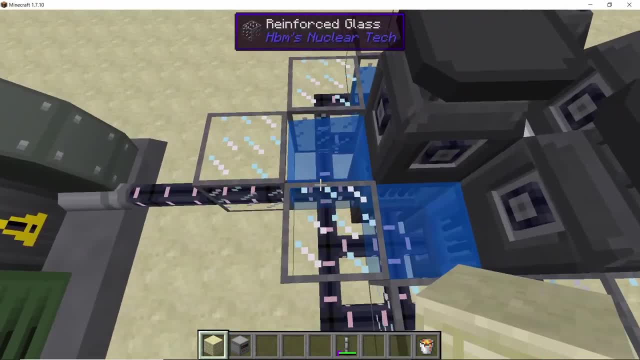 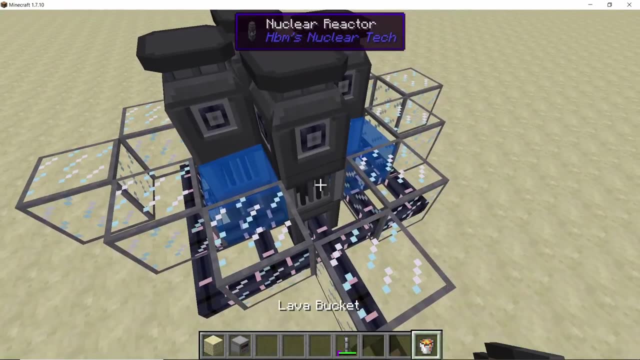 But the one that we are going to use is LAVA. So, like the one that we are going to use, So like the water that we have placed here, What happens if you place lava Now? the lava will help in increasing the hull temperature of your nuclear reactor. 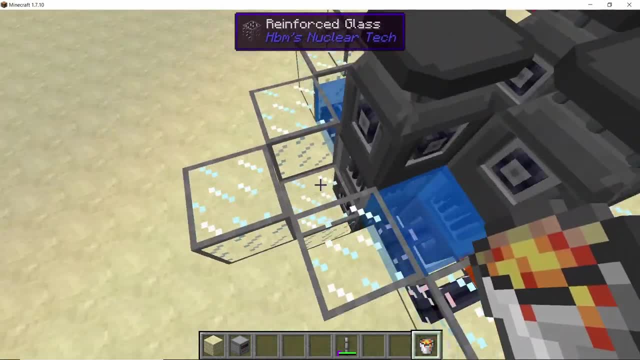 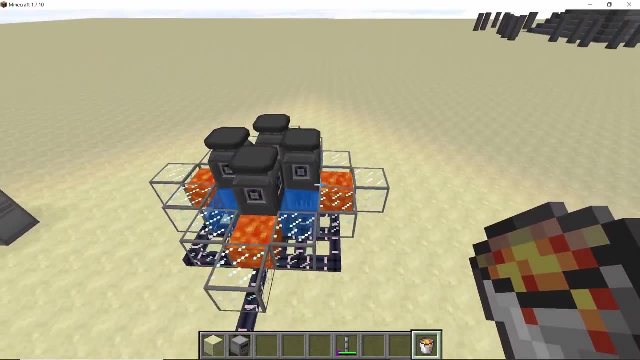 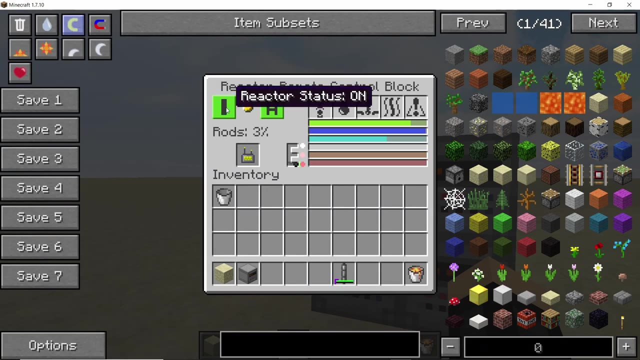 And, as you remember, I told you, hull is the place where water is kept. So if you raise the hull temperature, it will increase the production of steam, and increased production of steam means more energy. So now let's start off the reaction, And there 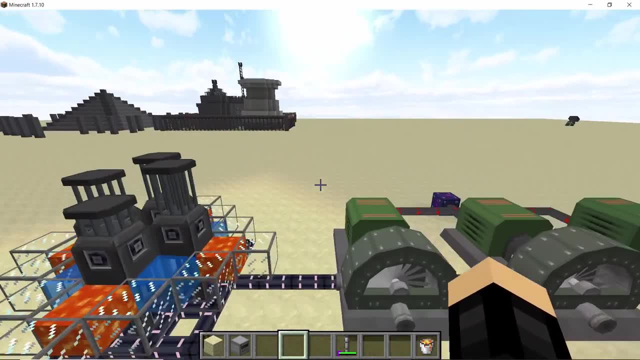 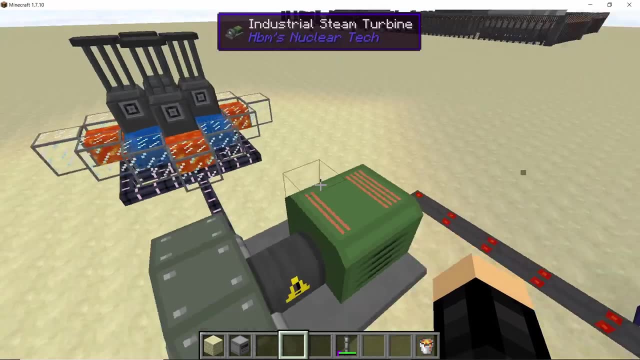 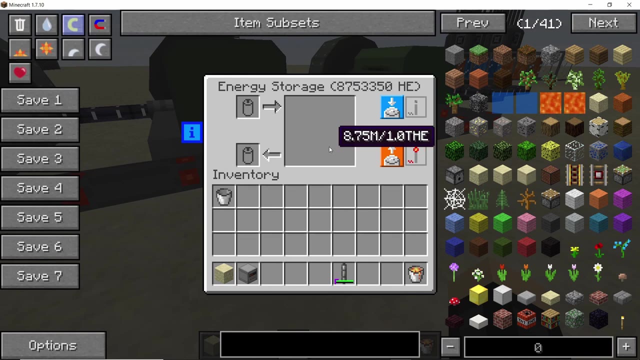 Okay, so now that all the control rods are up, let's see what is the amount of energy that we are getting, whether it is more or less. And look at this: If you remember correctly, previously our setup was not moving at this fast speed. 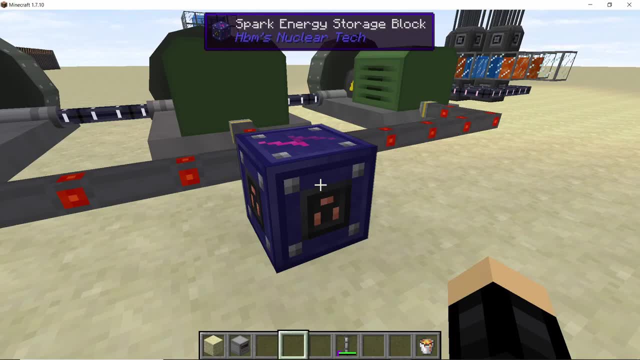 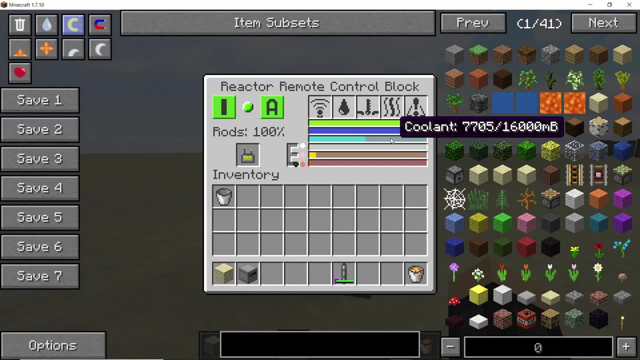 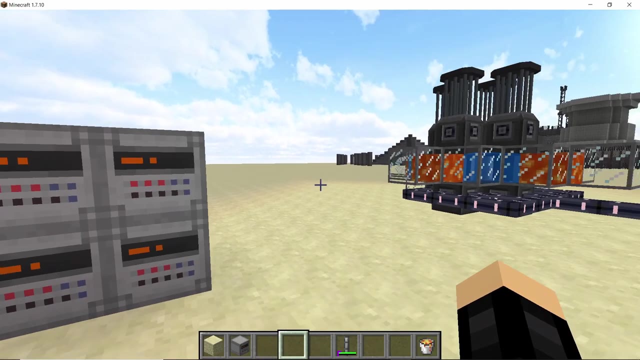 And now look at the rate of energy production. So this is how. this is one example of how you can use modifiers, But there are a lot of modifiers available, So experiment yourself and try them out. They are really interesting, guys. And, as you can see, the hull heat has gone up to 86 degrees from the previous 46 degrees. 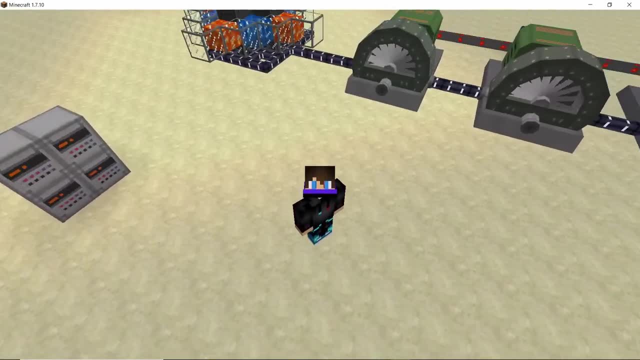 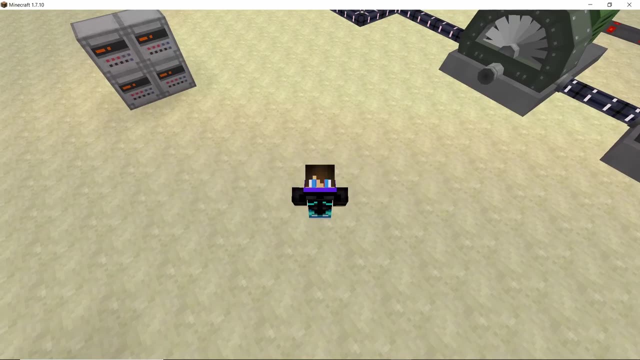 So that was all I had for this video, guys. If you guys like this detailed review, please smash that like button and also subscribe to my channel. If you want to see more tutorials like this in the future, let me know in the comment. 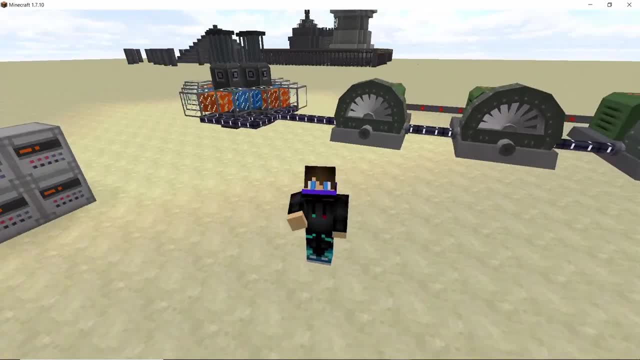 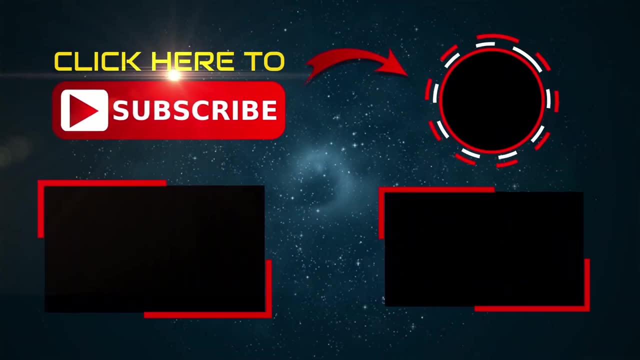 section down below how you found this video and ideas for any future video. Peace out, guys. Stay safe, Bye, Bye, Bye, Bye, Bye.